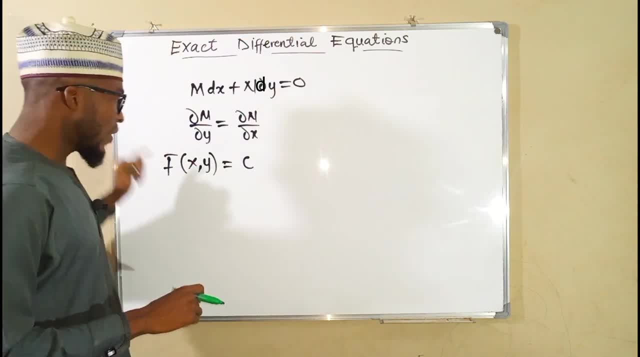 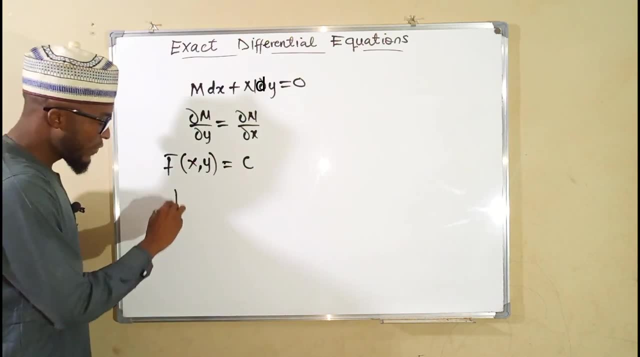 constant to find the total derivative of this function. let us apply the general constant to find the total derivative of this function. let us apply the general Chan rule, which says that, and the derivative of this function of this Chan rule, which says that, and the derivative of this function of this. 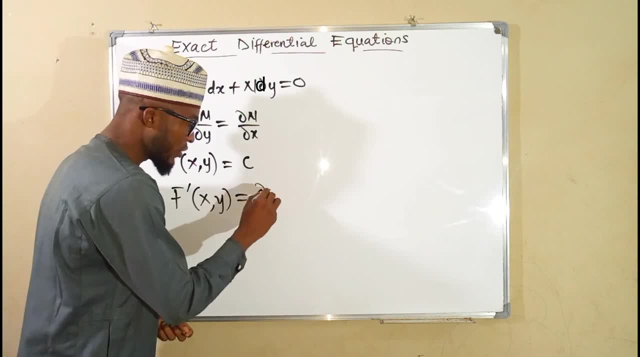 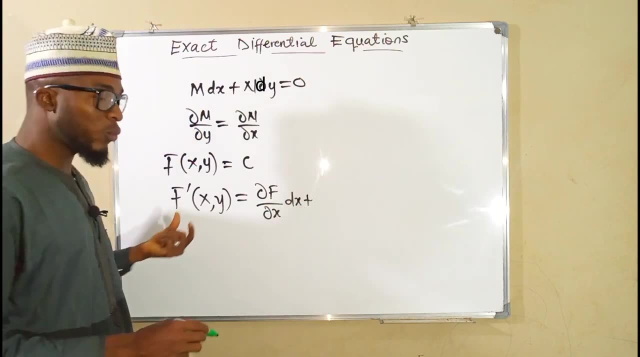 infelicit function is going to be partial derivative of F with respect to infelicit function is going to be partial derivative of F. with respect to X DX. then we add: we now differentiate the function with respect to Y partial X DX. then we add: we now differentiate the function with respect to Y- partial. derivative of F with respect to X. then we add: we now differentiate the function with respect to Y- partial derivative of F with derivative of F with respect to X. then we add: we now differentiate the function with: derivative of F with respect to Y- partial derivative of F with respect to Y- partial. 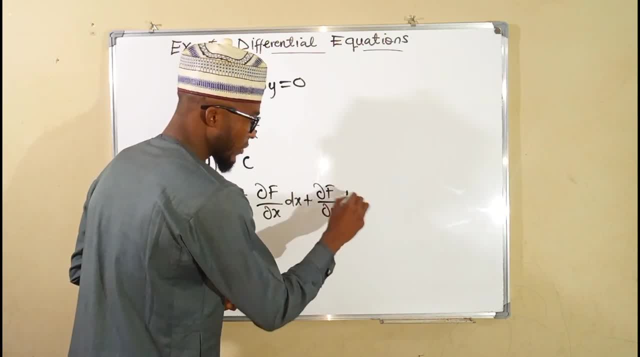 derivative of F with respect to Y, partial respect to Y dy, and this is equal to respect to Y dy, and this is equal to respect to Y dy, and this is equal to remember. if you differentiate a constant, remember. if you differentiate a constant, remember. if you differentiate a constant, you definitely have to often, and zero. so 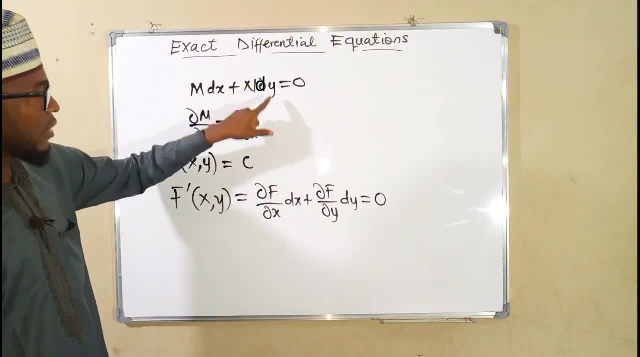 you definitely have to often and zero. so you definitely have to often and zero, so this is zero. so now, by relating this, this is zero. so now, by relating this, this is zero. so now, by relating this equation and this equation, you can see equation and this equation you can see. 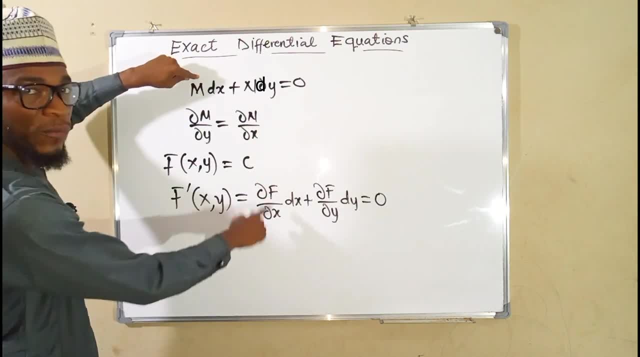 equation. and this equation, you can see that M correspond to the partial, that M correspond to the partial, that M correspond to the partial derivative of F with respect to X. so we derivative of F with respect to X, so we derivative of F with respect to X. so we can see M is equal to the partial. 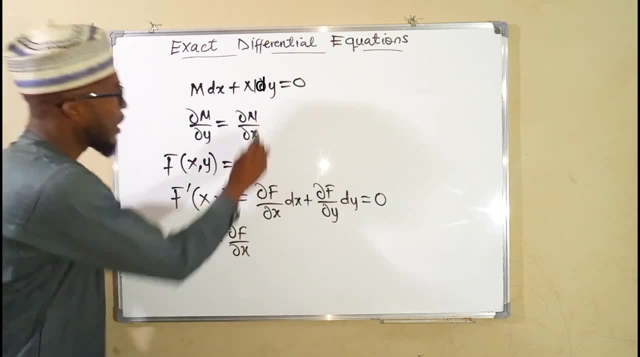 can see: M is equal to the partial. can see: M is equal to the partial derivative of F with respect to X and N. derivative of F with respect to X and N. derivative of F with respect to X and N. correspond to the partial derivative F correspond to the partial derivative F. 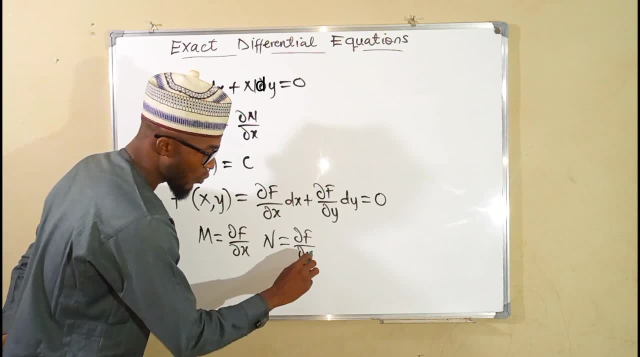 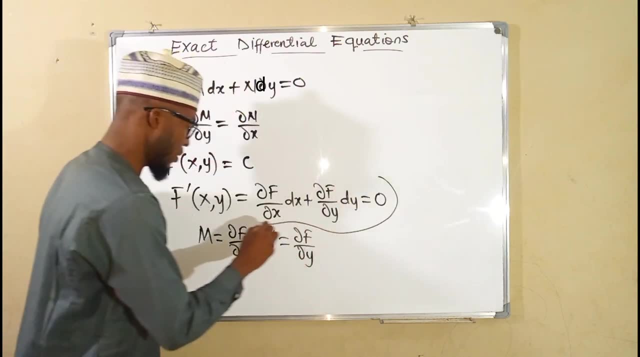 correspond to the partial derivative F with respect to 2y. so the question is with respect to 2y, so the question is with respect to 2y. so the question is: how can we solve this equation to? how can we solve this equation to: how can we solve this equation to obtain back our original function, this? 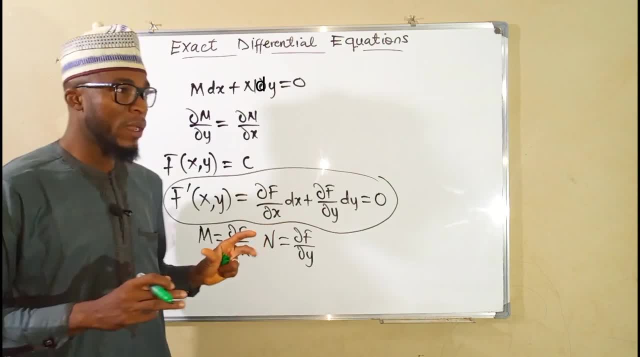 obtain back our original function. this obtain back our original function. this is what I will show you today. so in is what I will show you today. so in is what I will show you today. so, in order to understand this clearly, let me order to understand this clearly, let me. 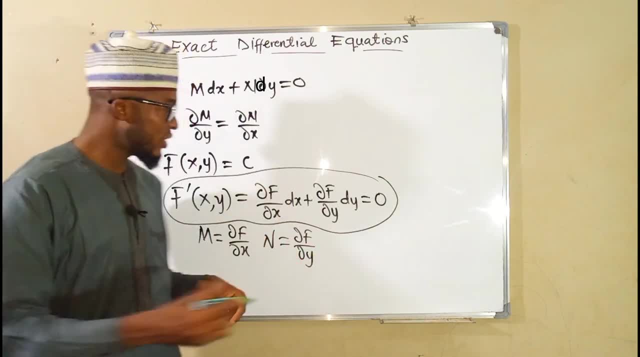 order to understand this clearly, let me bring an implicit function differentiated, bring an implicit function differentiated, bring an implicit function differentiated to obtain this form of equation. and see to obtain this form of equation. and see to obtain this form of equation and see how we can solve it back to obtain our 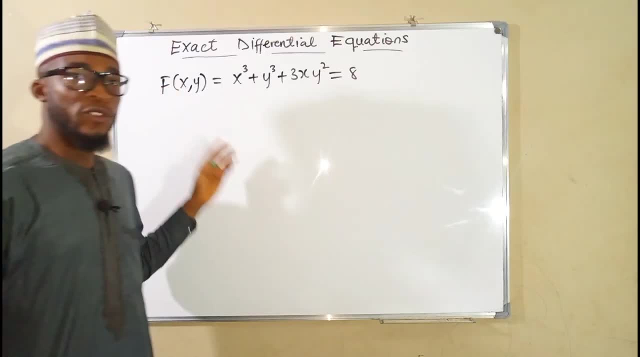 how we can solve it back to obtain our, how we can solve it back to obtain our initial function. suppose this is our initial function. suppose this is our initial function. suppose this is our implicit function. to differentiate it: implicit function. to differentiate it: implicit function. to differentiate it using the total derivative we have to 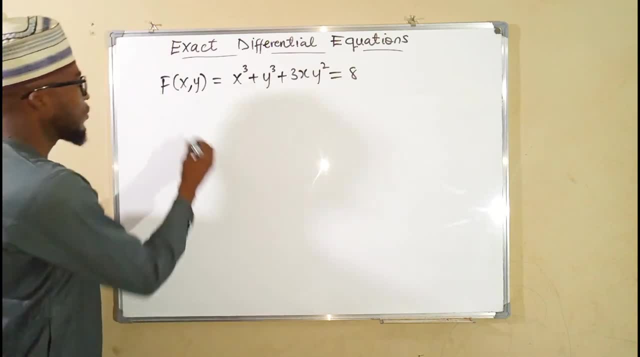 using the total derivative, we have to. using the total derivative, we have to apply the general chain rule, which is F. apply the general chain rule, which is F. apply the general chain rule, which is F. prime of this function, X, some Y and prime of this function X, some Y. and. 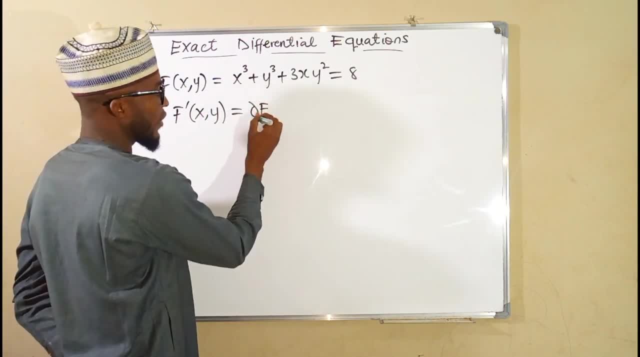 prime of this function X, some Y, and you know it is going to be the partial. you know it is going to be the partial. you know it is going to be the partial derivative of F with respect to X- DX. derivative of F with respect to X- DX. 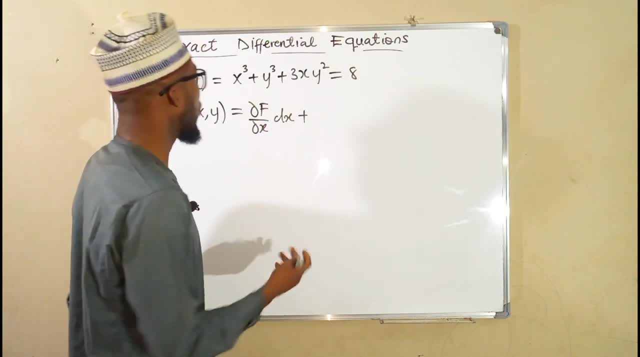 derivative of F with respect to X, DX. plus we differentiate the function again, plus we differentiate the function again, plus we differentiate the function again with respect to Y. we have to take the with respect to Y. we have to take the with respect to Y. we have to take the partial derivative of F with respect to. 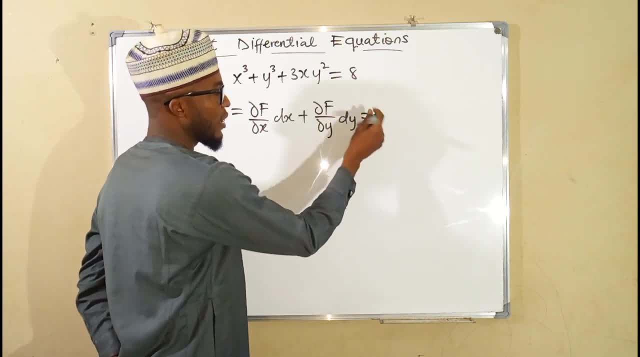 partial derivative of F with respect to partial derivative of F with respect to Y- dy. and you know, by differentiating if y, dy. and you know by differentiating if y, dy. and you know by differentiating if constant. we have to get zero, so now let constant. we have to get zero, so now let. 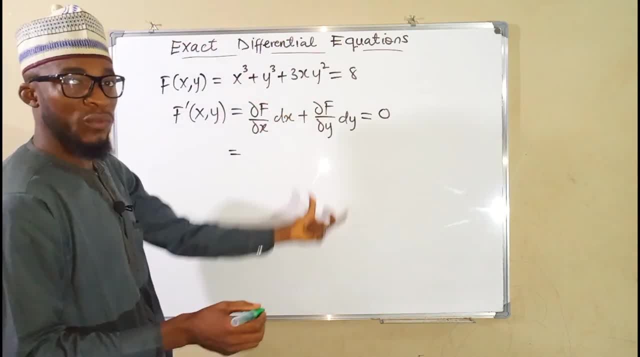 constant, we have to get zero. so now let us substitute. this is equal to anywhere. us substitute. this is equal to anywhere. us substitute. this is equal to anywhere we have X, we have to differentiate. we have X, we have to differentiate. we have X, we have to differentiate, treating Y as constant. so this becomes: 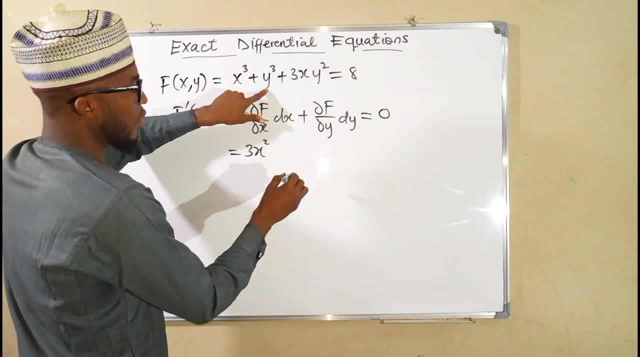 treating Y as constant. so this becomes treating Y as constant. so this becomes 3 X to the second power. this is constant. 3 X to the second power, this is constant. 3 X to the second power: this is constant. it becomes 0. we move here, we treat every. 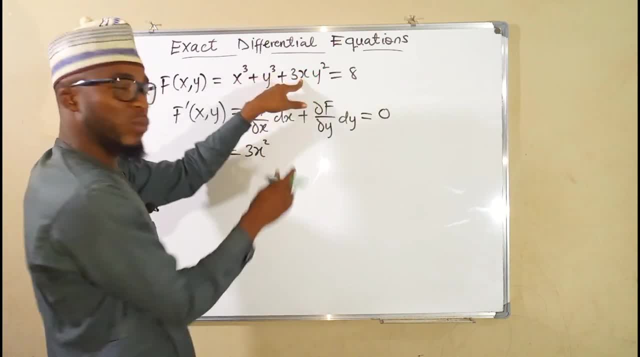 it becomes 0, we move here. we treat every. it becomes 0, we move here. we treat every other term as constant except X. so other term as constant except X, so other term as constant except X. so differentiating X, we get 1, we have 3 Y. 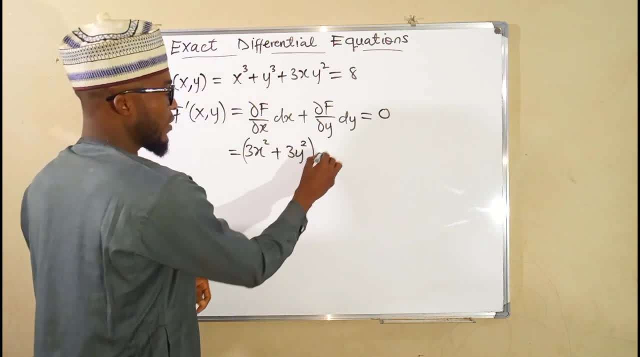 differentiating X: we get 1. we have 3 Y. differentiating X: we get 1. we have 3 Y squared left, and all this. we have DX squared left and all this. we have DX squared left and all this. we have DX. then plus we differentiate the function. 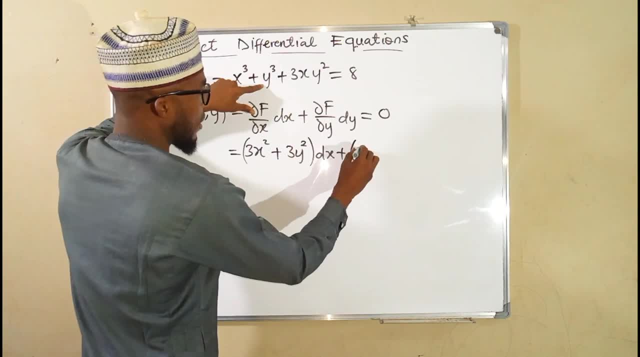 then plus we differentiate the function, then plus we differentiate the function again with respect to Y, because you, what? again with respect to Y, because you, what? again with respect to Y, because you, what we have here as 3 Y to the second power, we have here as 3 Y to the second power. 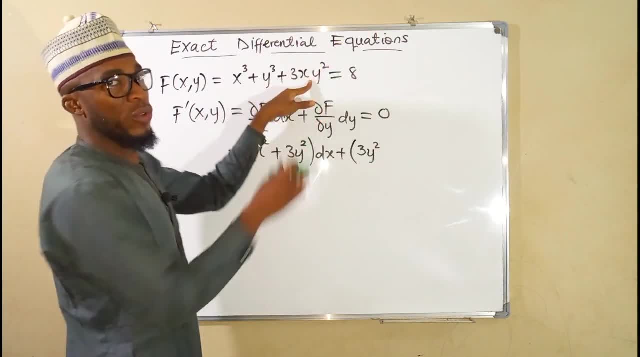 we have here as 3 Y to the second power. again, if you differentiate y, squared you again. if you differentiate y, squared you again. if you differentiate y squared, you are going to obtain 2y x 3x. you have to. are going to obtain 2y x 3x, you have to. 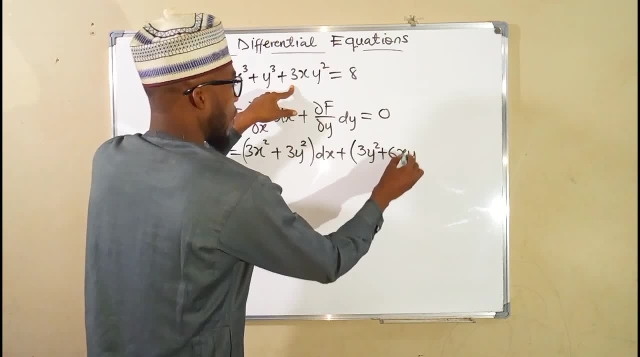 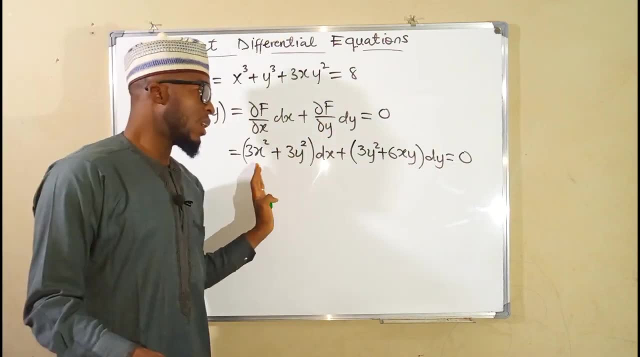 are going to obtain 2y x 3x. you have to obtain 6 X Y and we have dy and the obtain 6 X Y and we have dy and the obtain 6 X Y and we have dy, and the whole of this equal to 0. so this is the. 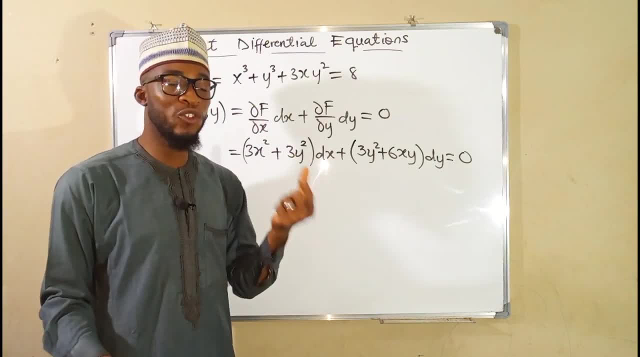 whole of this equal to 0. so this is the whole of this equal to 0. so this is the form of an exact differential equation, form of an exact differential equation, form of an exact differential equation, but we have to test whether it is really. but we have to test whether it is really. 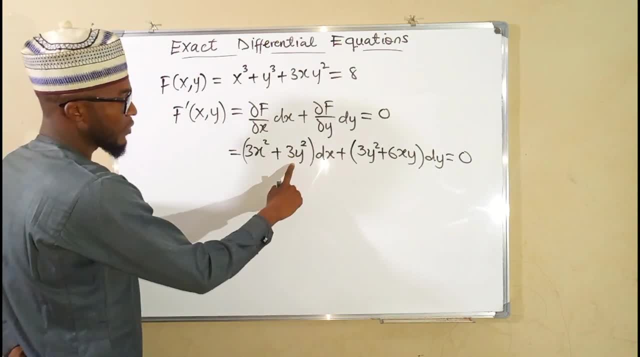 but we have to test whether it is really exact or not. remember this is our M, exact or not? remember this is our M, exact or not. remember this is our M, because we see the partial derivative of, because we see the partial derivative of, because we see the partial derivative of F with respect to X is equal to that. 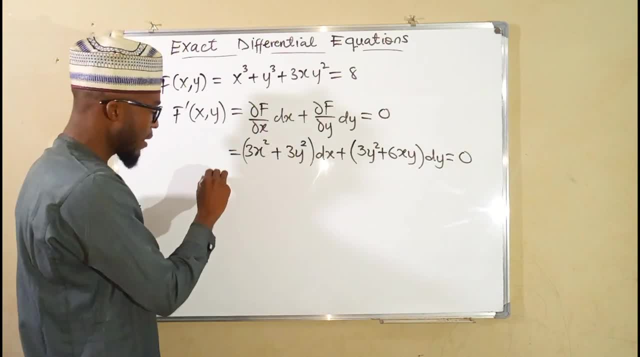 F with respect to X is equal to that. F with respect to X is equal to that time that is connected with DX. so we time that is connected with DX, so we time that is connected with DX. so we see M is equal to 3x squared plus 3y. 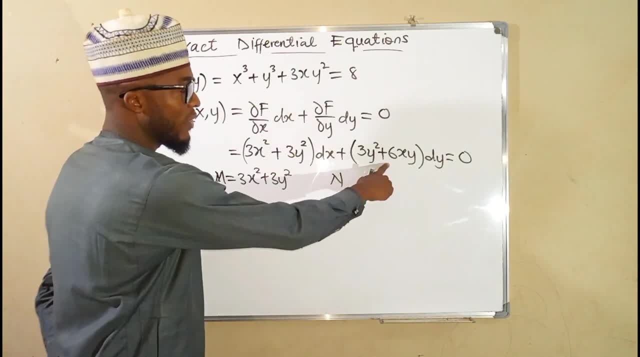 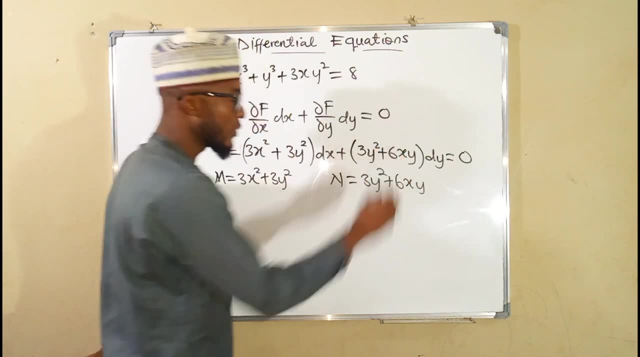 see M is equal to 3x squared plus 3y. see M is equal to 3x squared plus 3y squared, while n is going to be this squared, while n is going to be this squared, while n is going to be this times, equal to 3y squared plus 6x y. so 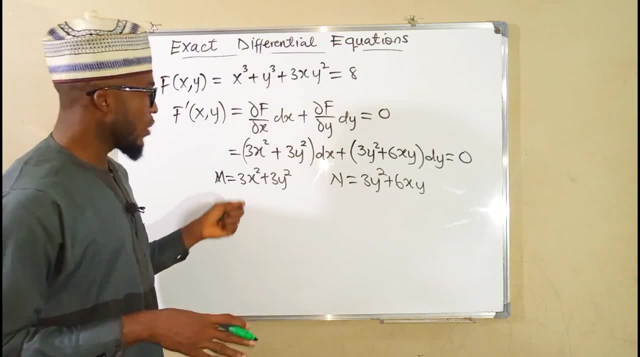 times equal to 3y squared plus 6x y. so times equal to 3y squared plus 6x y. so to testify whether it is an exact or not, to testify whether it is an exact or not. to testify whether it is an exact or not, we are going to differentiate this with. 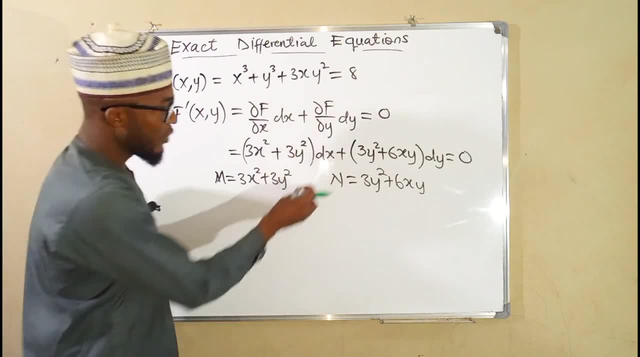 we are going to differentiate this with. we are going to differentiate this with respect to y. to understand this clearly. respect to y. to understand this clearly. respect to y. to understand this clearly. you can see the one that is attached to. you can see the one that is attached to. 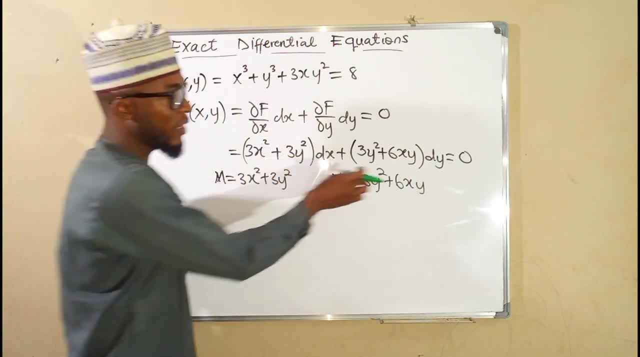 you can see the one that is attached to the X. you're going to differentiate it, the X. you're going to differentiate it, the X. you're going to differentiate it with respect to y, and that's that is with respect to y, and that's that is. 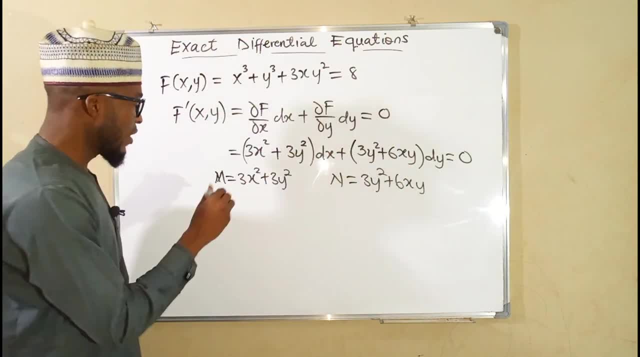 with respect to y, and that's that is connected to dy. you differentiate it connected to dy. you differentiate it connected to dy. you differentiate it with respect to X. so we say D partial with respect to X. so we say D partial with respect to X. so we say D partial derivative of M with respect to Y is: 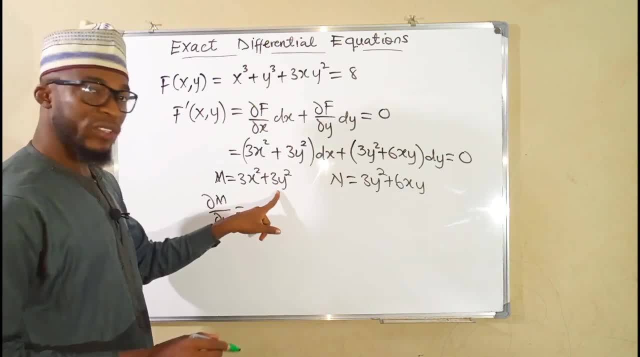 derivative of M with respect to Y is derivative of M with respect to Y is going to be. this is constant. if you going to be, this is constant. if you going to be, this is constant. if you differentiate this, you have 10: 6 y now. differentiate this, you have 10, 6 y now. 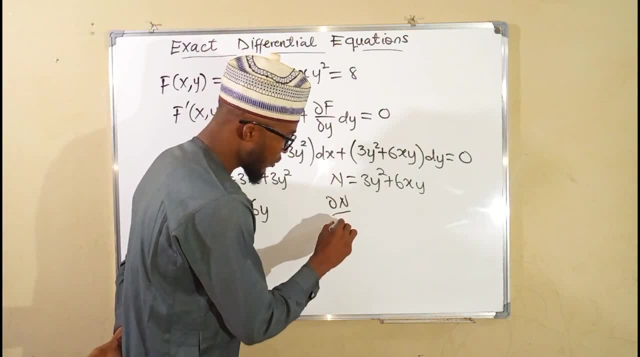 differentiate this. you have 10, 6 y. now we do the same thing here, we. we do the same thing here we. we do the same thing here. we. differentiate this n with respect to X, differentiate this n with respect to X. differentiate this n with respect to X alone, treating Y as constant. so this: 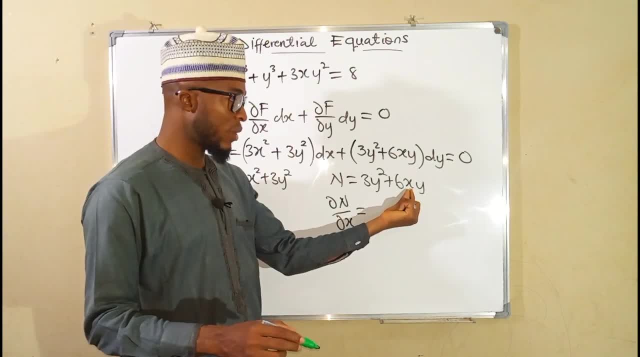 alone treating Y as constant. so this alone treating Y as constant. so this becomes constant. if you differentiate X becomes constant. if you differentiate X becomes constant. if you differentiate X- here you have 10, 1- then 1 times 6 times. here you have 10, 1, then 1 times 6 times. 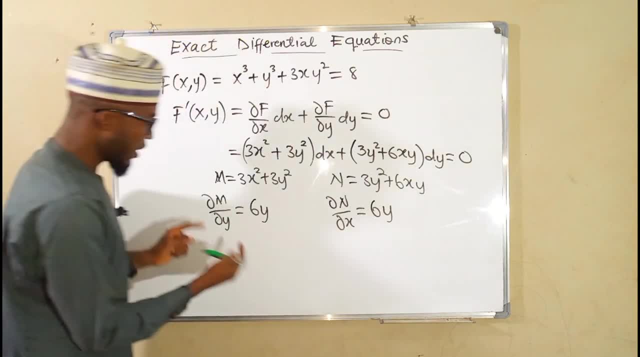 here you have 10, 1, then 1 times 6 times Y is 6. why you can see that the partial Y is 6. why you can see that the partial Y is 6. why you can see that the partial derivative of M with respect to Y is 6. 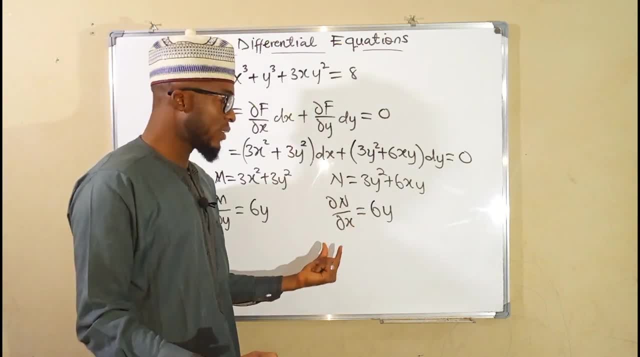 derivative of M with respect to Y is 6. derivative of M with respect to Y is 6. why I like. why the partial derivative of. why I like. why the partial derivative of. why I like. why the partial derivative of n with respect to X is also 6. why? 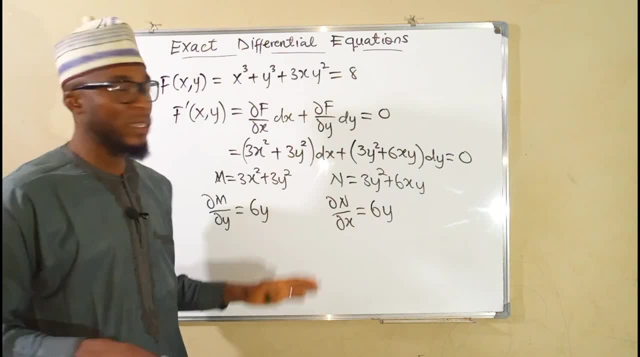 n with respect to X is also 6? why n with respect to X is also 6? why, since this is equal to this, we conclude: since this is equal to this, we conclude. since this is equal to this, we conclude by saying it is an exact differential. 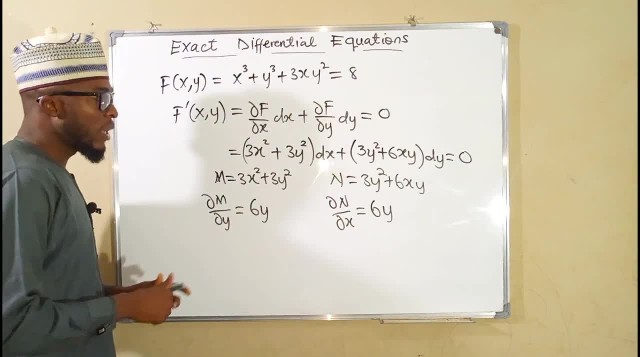 by saying it is an exact differential, by saying it is an exact differential equation, since it is an exact equation, since it is an exact equation, since it is an exact differential equation, let us find out how differential equation, let us find out how differential equation, let us find out how we can solve it from here, you can see. 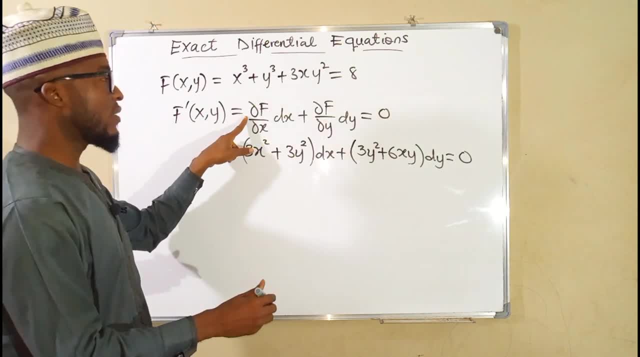 we can solve it from here. you can see. we can solve it from here. you can see that 3x y plus 3y squared is the same, that 3x y plus 3y squared is the same, that 3x y plus 3y squared is the same thing as the partial derivative of F. 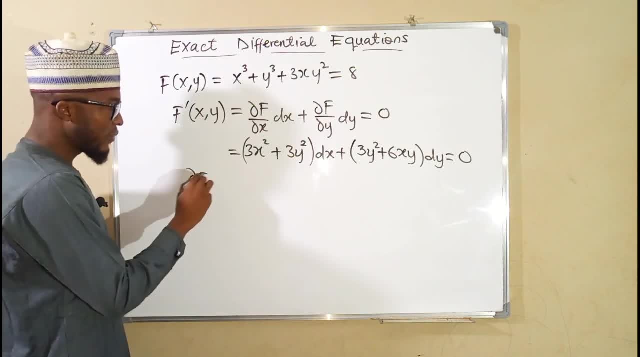 thing as the partial derivative of F, thing as the partial derivative of F with respect to X. so we have the partial with respect to X. so we have the partial with respect to X. so we have the partial derivative of F with respect to X. this is derivative of F with respect to X. this is. 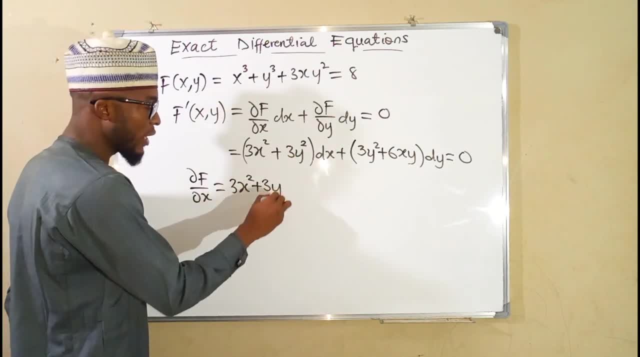 derivative of F with respect to X. this is equal to 3x squared plus 3y squared, equal to 3x squared plus 3y squared, equal to 3x squared plus 3y squared. now to obtain our original function, which. now to obtain our original function, which. 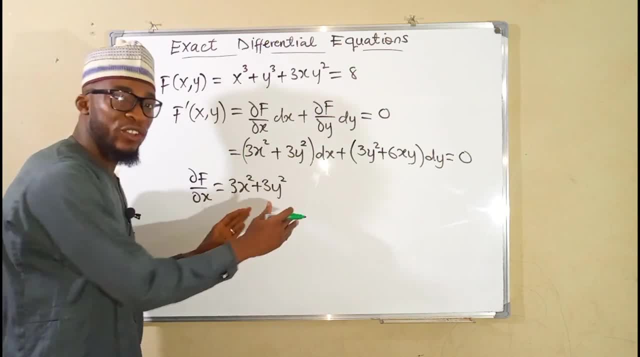 now to obtain our original function, which is this: we are going to integrate both is this: we are going to integrate both is this: we are going to integrate both sides of this equation with respect to X sides of this equation, with respect to X sides of this equation with respect to X. so we say, by integrating the left-hand. 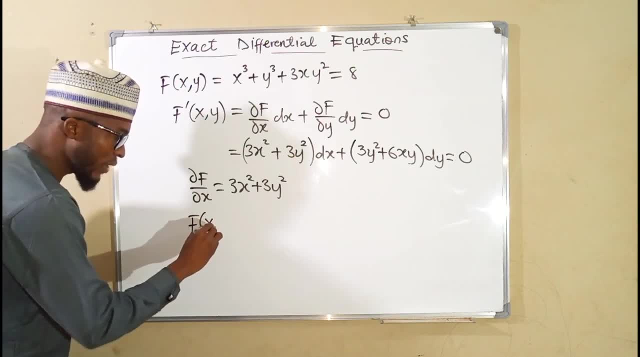 so we say: by integrating the left-hand, so we say: by integrating the left-hand side, we are going to obtain F, which is side. we are going to obtain F, which is side. we are going to obtain F, which is also a function of X and Y. this is equal. 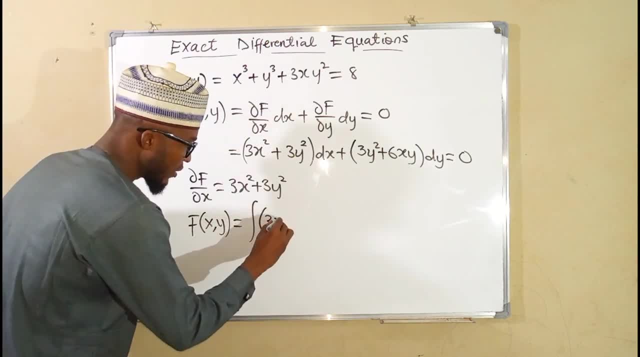 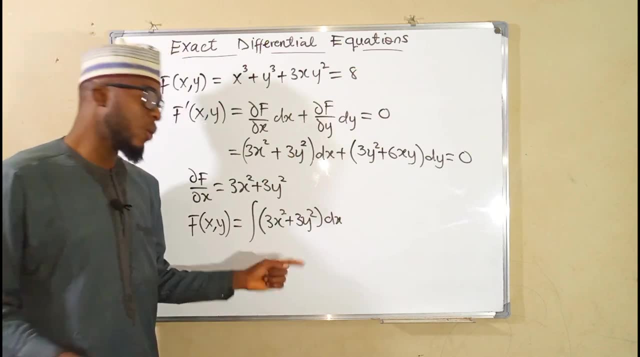 also a function of X and Y. this is equal, also a function of X and Y. this is equal to the integral of 3x squared plus 3y, to the integral of 3x squared plus 3y, to the integral of 3x squared plus 3y squared dx. well, remember, we are going to. 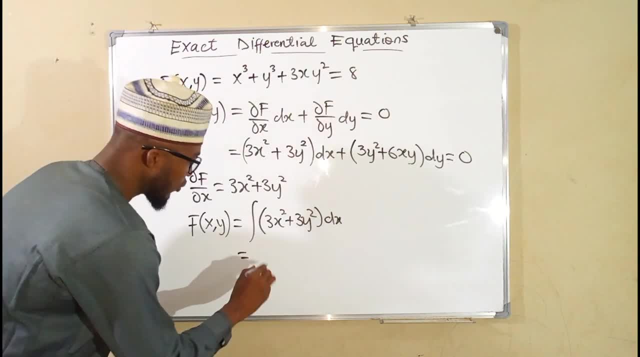 squared dx. well, remember, we are going to squared dx. well remember, we are going to treat Y as constant here. this is equal. treat Y as constant here: this is equal. treat Y as constant here, this is equal to. if you integrate this first time, the to. if you integrate this first time, the. 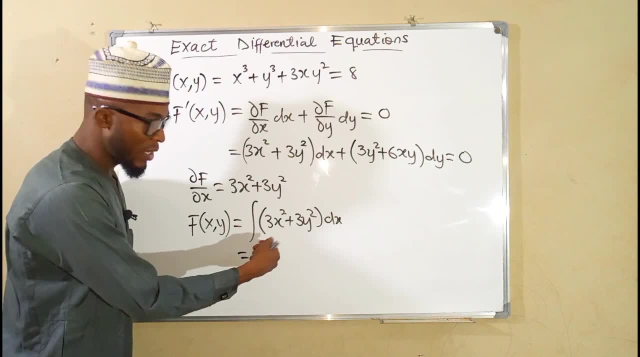 to. if you integrate this first time, the power has to increase by 1. make a tree: power has to increase by 1. make a tree: power has to increase by 1. make a tree: you have to divide by 3 that tree will. you have to divide by 3 that tree will. 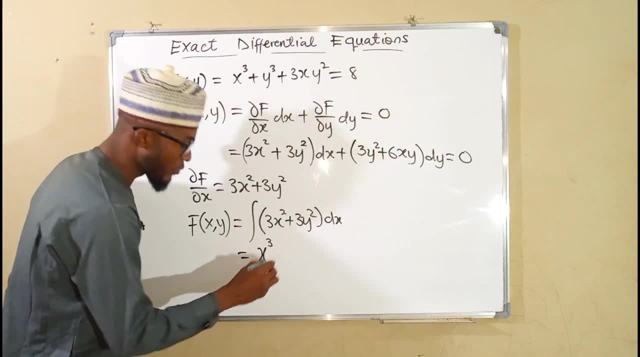 you have to divide by 3, that tree will cancel the study, leaving only X to the cancel the study, leaving only X to the cancel the study, leaving only X to the power of 3 plus all these are constants. power of 3 plus all these are constants. 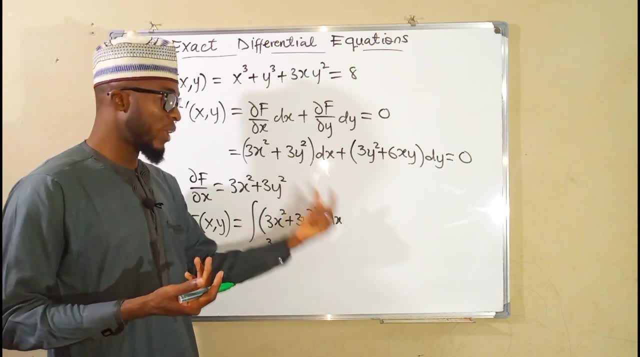 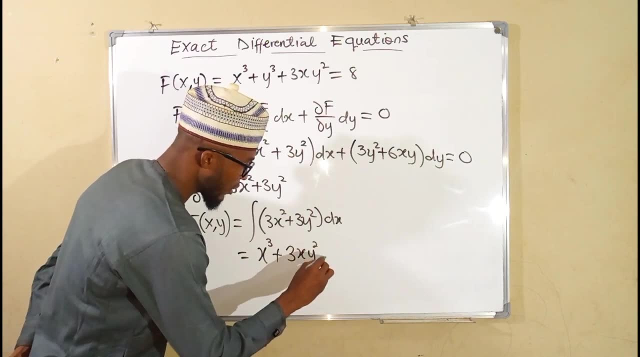 power of 3 plus. all these are constants. if you integrate a constant with respect, if you integrate a constant with respect, if you integrate a constant with respect to X, you just have to attach X to the to X. you just have to attach X to the to X, you just have to attach X to the constant. so we have 3, X, Y squared plus. 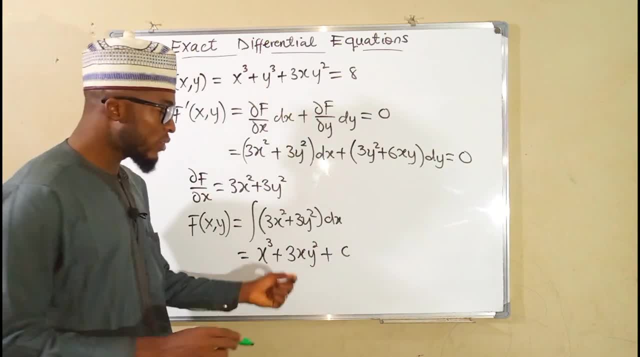 constant, so we have 3 X- Y squared plus constant, so we have 3 X- Y squared plus our constant of integration. but that, our constant of integration, but that our constant of integration. but that constant must be with respect to Y, constant must be with respect to Y. 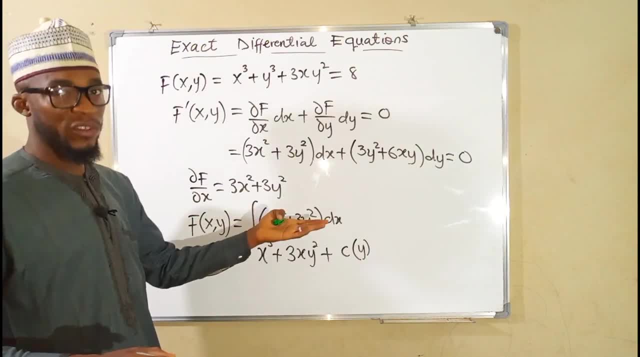 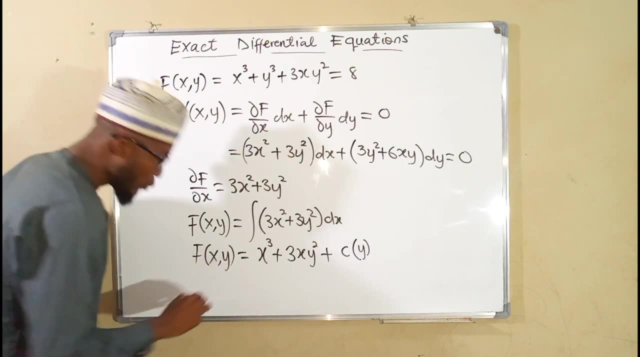 constant must be with respect to Y, because we treated Y as constant in, because we treated Y as constant in, because we treated Y as constant in this expression. so this is our original, this expression, so this is our original, this expression, so this is our original function. but our original function does. 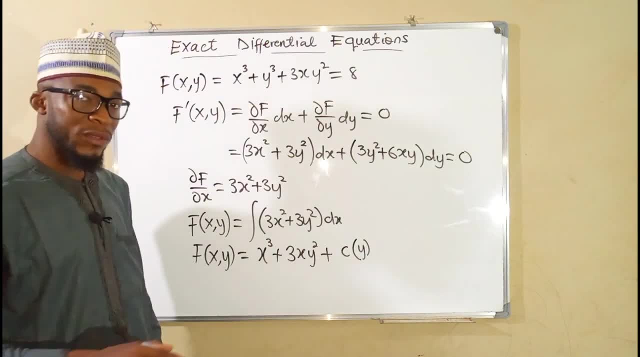 function, but our original function does function. but our original function does not contain C of Y. so how can we, if you not contain C of Y? so how can we if you not contain C of Y? so how can we, if you go out, what exactly the C of Y is? 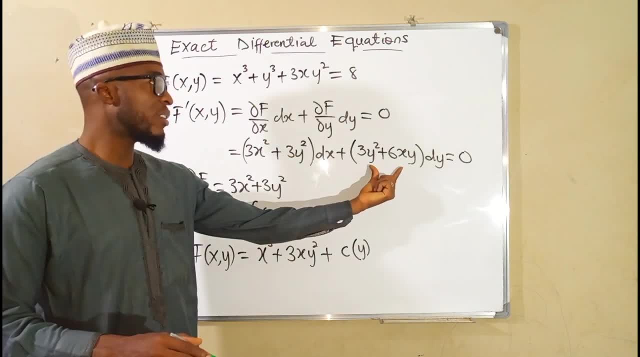 go out what exactly the C of Y is. go out what exactly the C of Y is. remember. this is a partial derivative of remember. this is a partial derivative of remember. this is a partial derivative of F with respect to Y. therefore we can F with respect to Y, therefore we can. 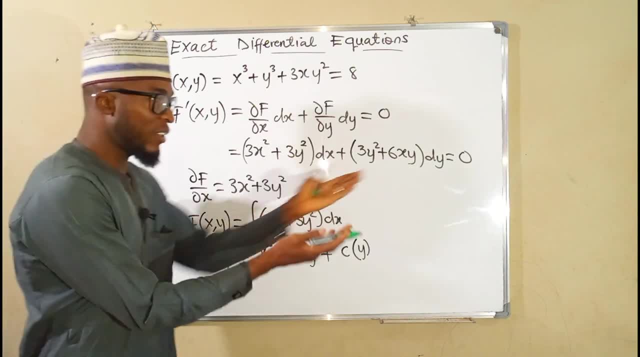 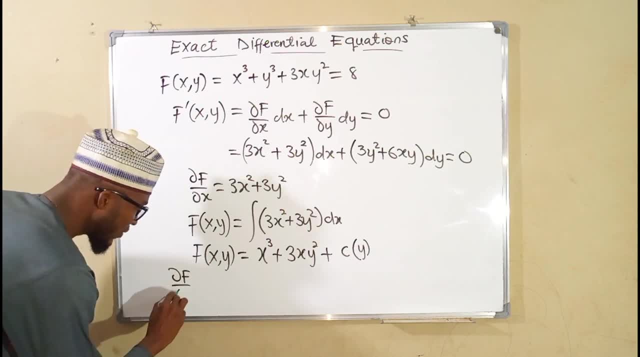 I relate the two functions. so let's do that partial derivative of F with that partial derivative of F, with that partial derivative of F with respect to Y, which is this: we are going respect to Y, which is this: we are going respect to Y, which is this: we are going to treat X as constant. therefore this: 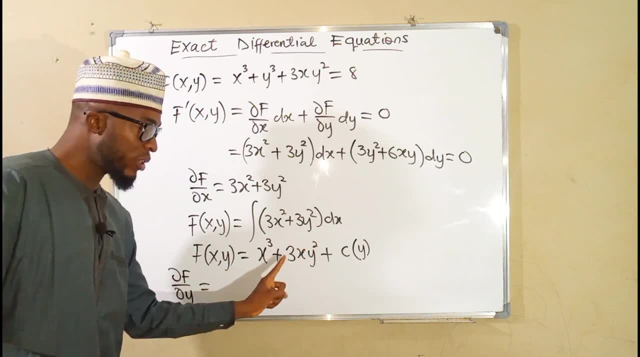 to treat X as constant, therefore this: to treat X as constant, therefore, this becomes 0. if you differentiate this just becomes 0. if you differentiate this just becomes 0. if you differentiate this just to multiply by 3, we have 6: X, Y and 2. 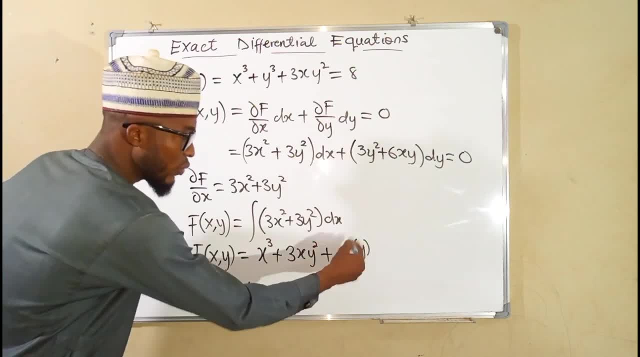 to multiply by 3, we have 6 X- Y and 2. to multiply by 3, we have 6 X, Y and 2 reduced by 1 plus. this is also a term reduced by 1 plus. this is also a term reduced by 1 plus. this is also a term with respect to Y, so we have to. 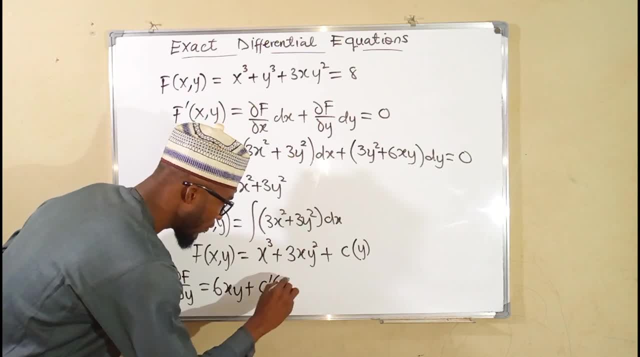 with respect to Y, so we have to. with respect to Y, so we have to differentiate it. we have C prime of Y. it differentiate it. we have C prime of Y. it differentiate it. we have C prime of Y. it means that this function must be, means that this function must be. 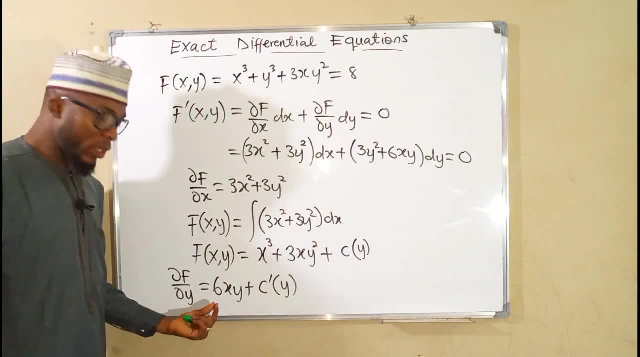 means that this function must be exactly as this. you can see, we have 6 X Y. exactly as this. you can see, we have 6 X Y. exactly as this. you can see: we have 6 X Y here. we equally have 6 X Y here. this: 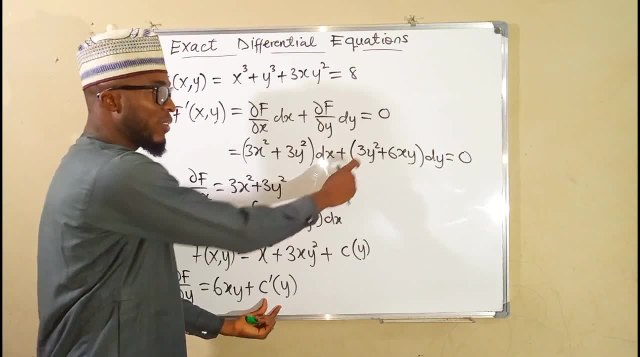 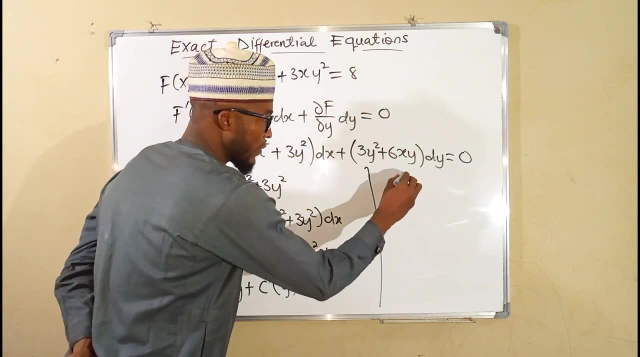 here we equally have 6 X Y here. this: here we equally have 6 X Y here. this means that C prime of Y must be equal, means that C prime of Y must be equal, means that C prime of Y must be equal to this 3y squared. so we say C prime of Y. 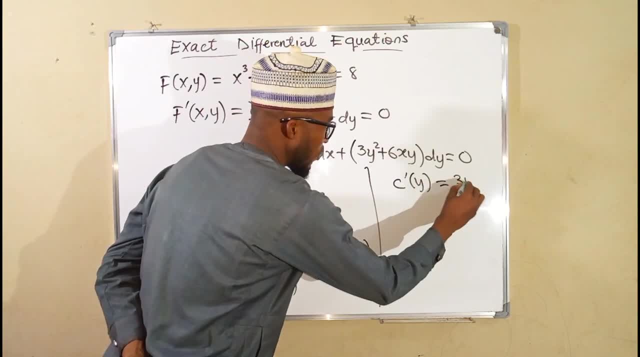 to this 3y squared. so we say C prime of Y. to this 3y squared. so we say C prime of Y is equal, is equal, is equal to this 3y squared. but what we are looking to, this 3y squared, but what we are looking, 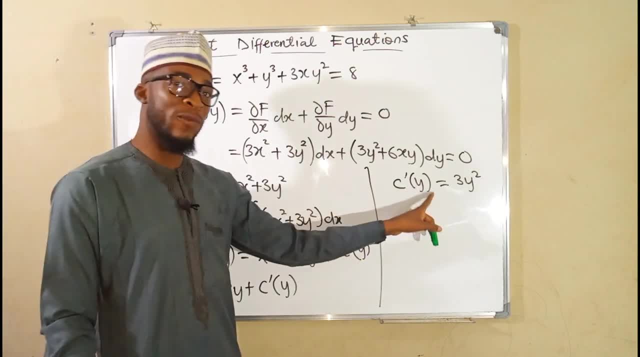 to this 3y squared. but what we are looking for to complete our function is C of Y, for to complete our function is C of Y. for to complete our function is C of Y, not C prime of Y. therefore we are going, not C prime of Y. therefore we are going. 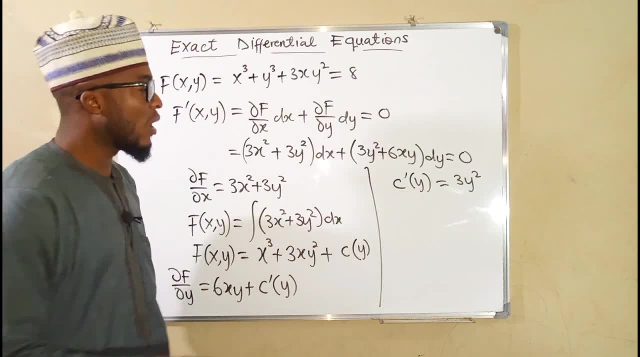 not C prime of Y. therefore, we are going to integrate both sides with respect to, to integrate both sides with respect to, to integrate both sides with respect to Y. so, by integrating this side with Y, so by integrating this side with Y, so by integrating this side with respect to Y, we're going to obtain only: 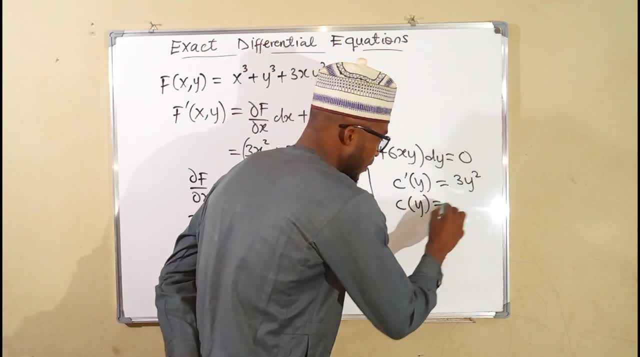 respect to Y. we're going to obtain only respect to Y. we're going to obtain only C of Y, and this is equal to the C of Y, and this is equal to the C of Y, and this is equal to the integral of 3y squared. with respect to Y: 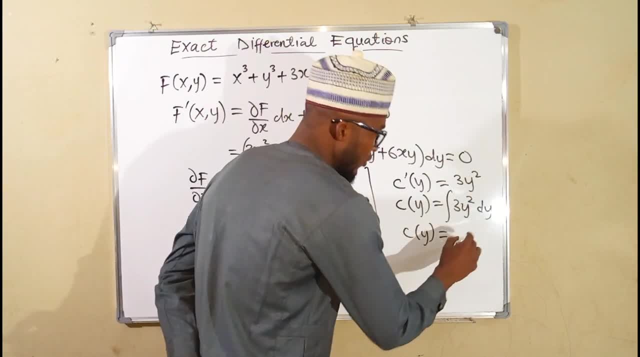 integral of 3y squared with respect to Y. integral of 3y squared with respect to Y. C of Y now will become equal to this. C of Y now will become equal to this. C of Y now will become equal to this. power will increase by 1, making 3 you. 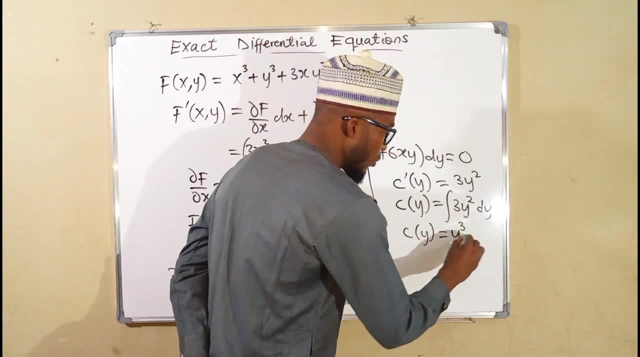 power will increase by 1 making 3. you power will increase by 1 making 3. you divide by 3, you obtain y to the third. divide by 3, you obtain y to the third. divide by 3, you obtain y to the third power, plus another constant of. 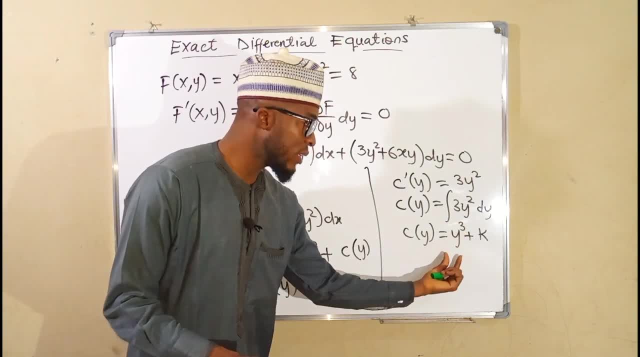 power plus another constant of power, plus another constant of integration. so we are going to integration, so we are going to integration. so we are going to substitute y to the third power plus K, substitute y to the third power plus K, substitute y to the third power plus K in this main function to obtain our 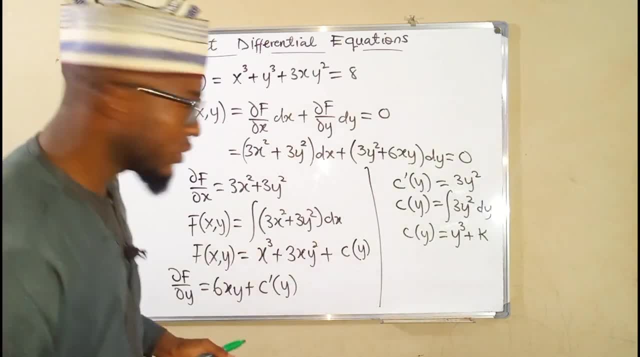 in this main function to obtain our, in this main function to obtain our general solution. so now let's do that by general solution. so now let's do that by general solution. so now let's do that by substitution. so now our function of X and substitution. so now our function of X, and 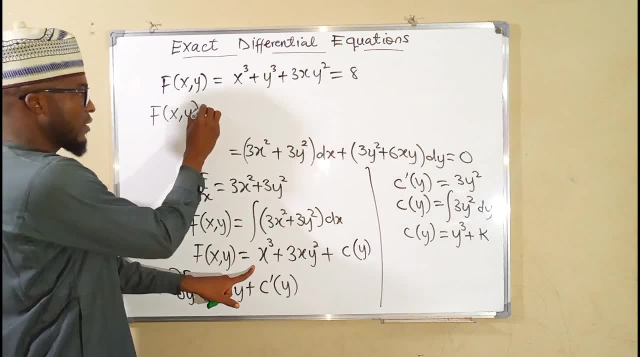 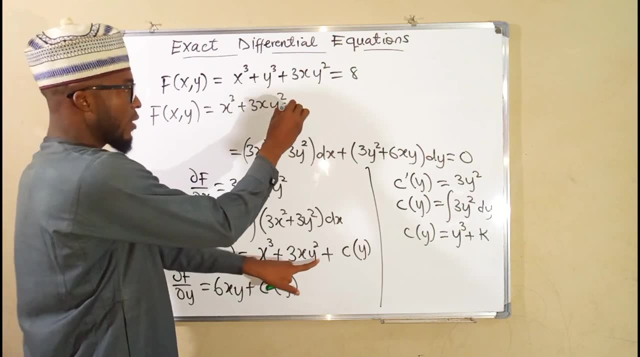 substitution. so now our function of X and Y, which is: this is equal to X to the Y, which is: this is equal to X to the Y, which is: this is equal to X to the third power plus 3x to the second power. third power plus 3x to the second power. 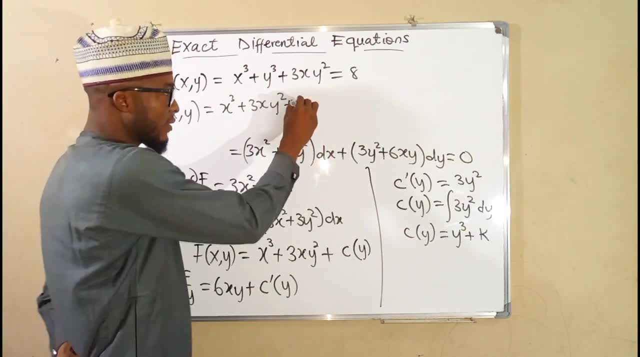 third power plus 3x to the second power plus C of Y, which we have here as Y, to plus C of Y, which we have here as Y, to plus C of Y, which we have here as Y, to the third power plus K, our original. the third power plus K, our original. 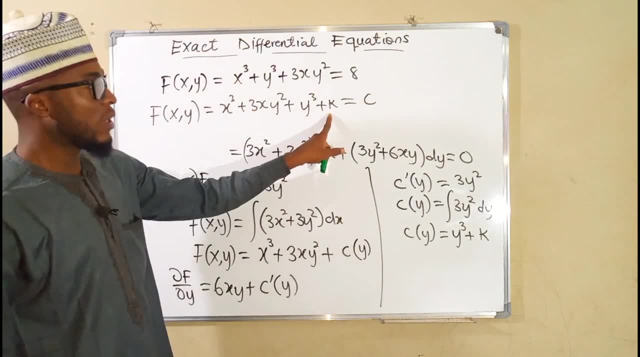 the third power plus K. our original function is equal to some. certain function is equal to some. certain function is equal to some certain constants, and you can see we have constants, and you can see we have constants, and you can see we have another constant here which we can. 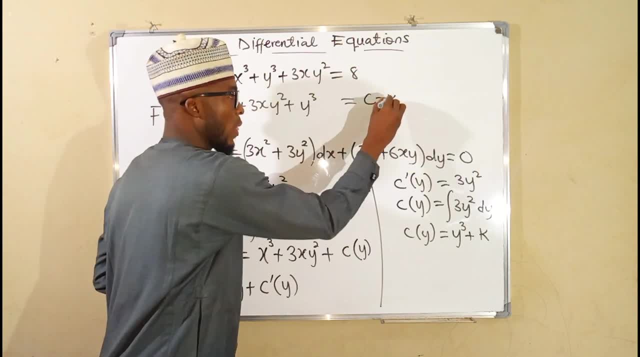 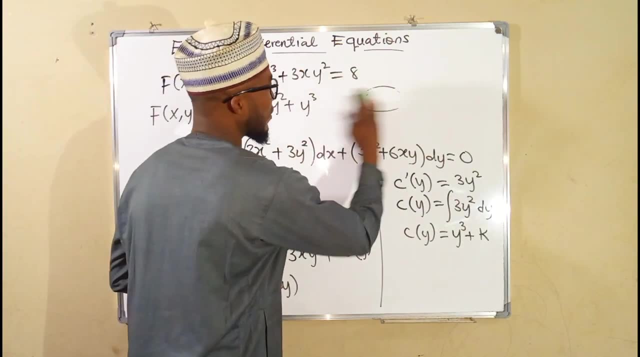 another constant here which we can, another constant here, which we can directly remove it from here and here, directly remove it from here and here, directly remove it from here and here. and a constant subtracting a constant is, and a constant subtracting a constant is, and a constant subtracting a constant is also a constant. so we can leave it as. 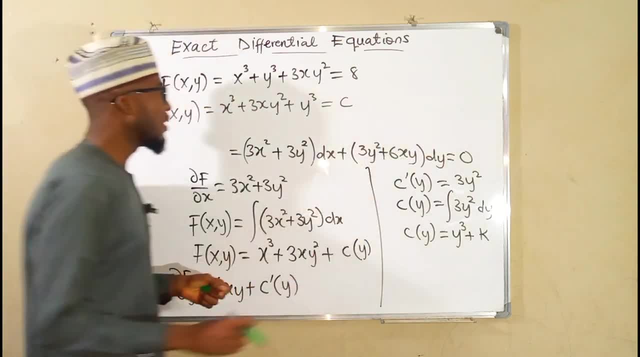 also a constant. so we can leave it as also a constant, so we can leave it as equal to some certain constant. so now, by equal to some certain constant, so now by equal to some certain constant. so now, by relating, you can see, we have X to the 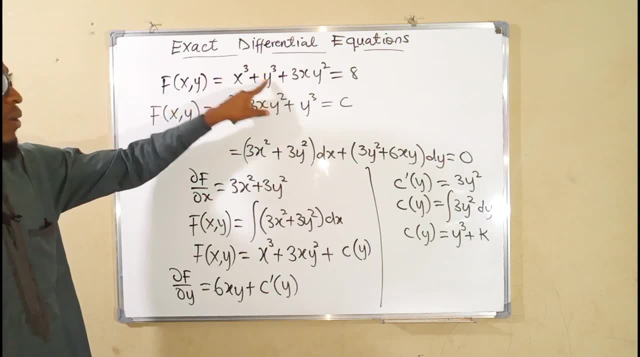 relating. you can see we have X to the relating. you can see we have X to the third power: here, we equally have it here. third power, here, we equally have it here. third power, here, we equally have it here. Y to the third power is also here, you. 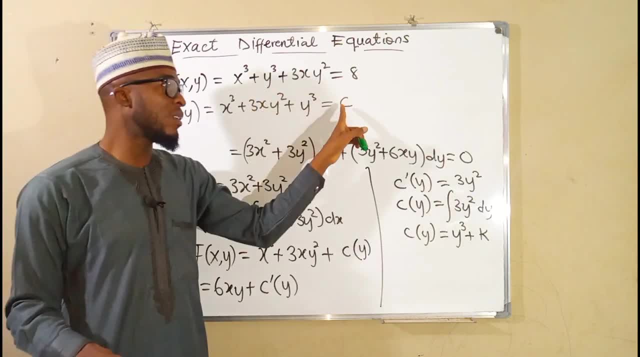 Y to the third power is also here. you. Y to the third power is also here. you can see we have a constant here. suppose can see we have a constant here. suppose can see we have a constant here. suppose we are given an initial condition, we, we are given an initial condition, we. 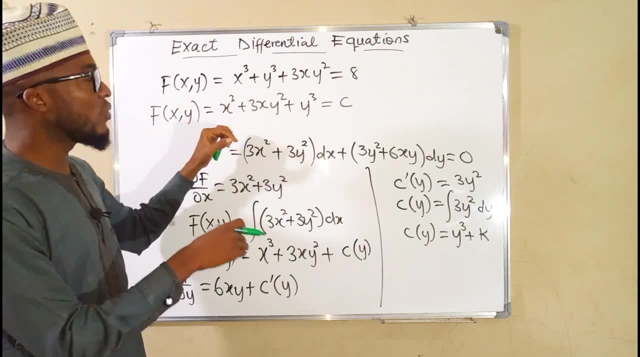 we are given an initial condition: we can substitute the values of Y and X back. can substitute the values of Y and X back. can substitute the values of Y and X back. to substitute an of 10, the. to substitute an of 10, the. to substitute an of 10, the corresponding value of C, which is 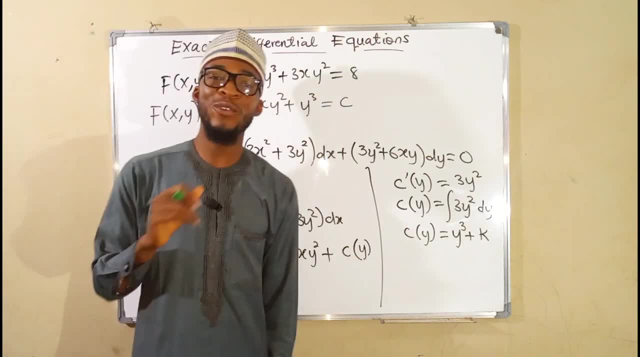 corresponding value of C, which is corresponding value of C, which is definitely has to be equal to it, so definitely has to be equal to it, so definitely has to be equal to it. so this is all I have for you today, thank. this is all I have for you today, thank. this is all I have for you today. thank you for watching. do have a nice day. 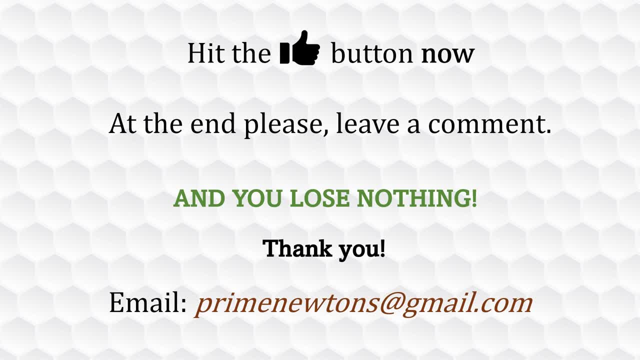 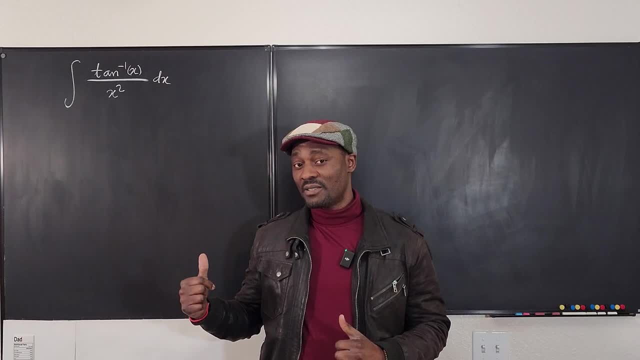 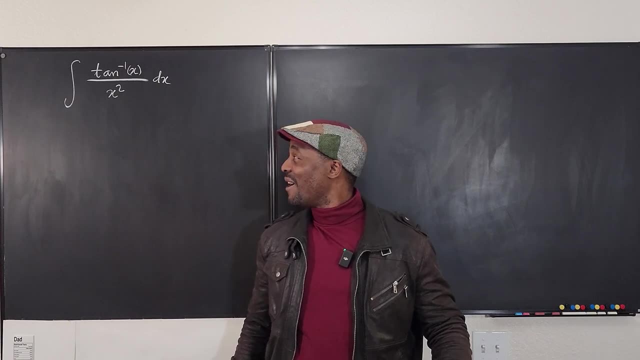 Hello, welcome to another video. Taking this integral might be a challenge, but if you start from what you know, it might take you to where you're supposed to be. So what can we do? I look at this and I go. 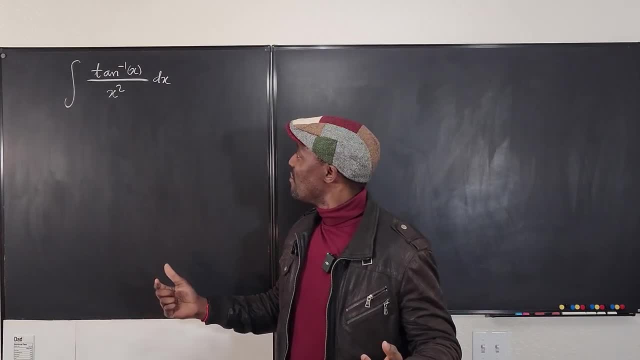 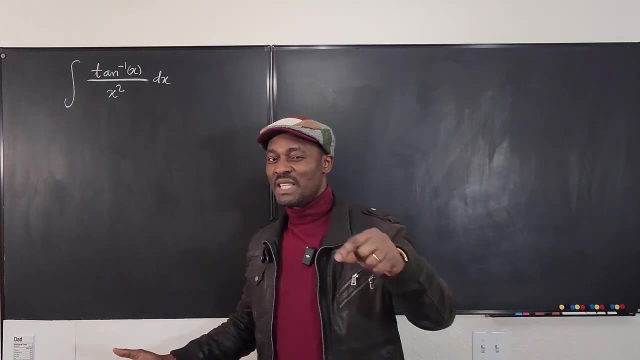 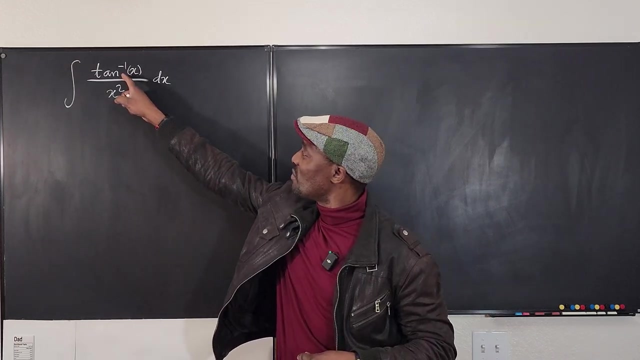 I can't do u-substitution or anything. Maybe I can do u-substitution, but it's not really a u-substitution because the derivative doesn't solve our problems, but it leads us in the path of a solution. So let's make u to be equal to r-tan of x and let's see what we.